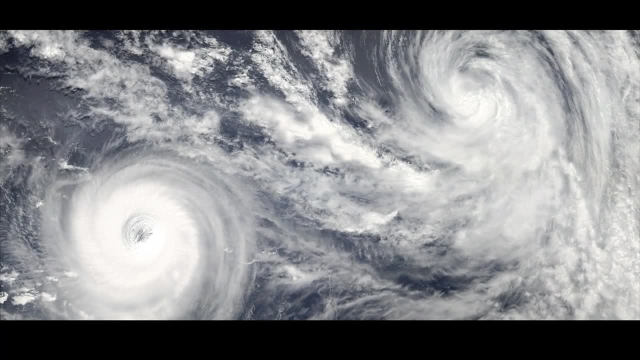 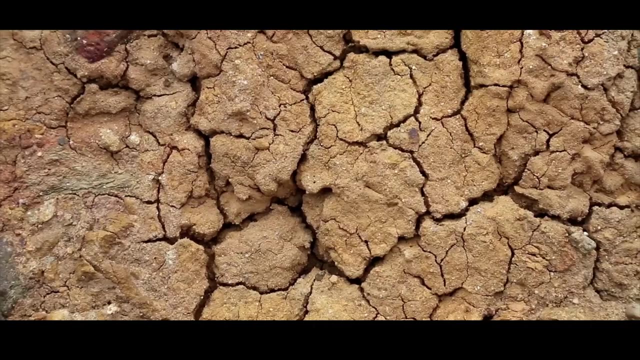 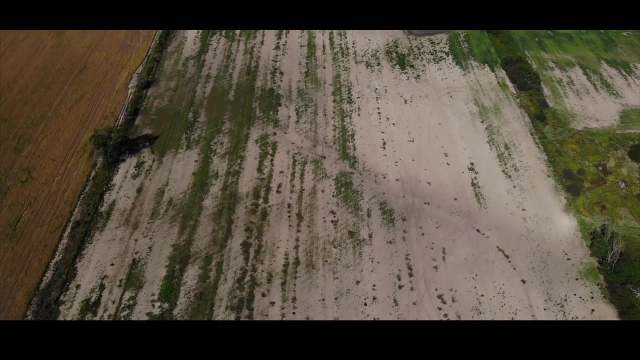 That exacerbates climate change, which results in extreme weather conditions and consequently requires more energy and water to grow our crops on land that is becoming increasingly stressed. Of course, irresponsible farming is not the only problem. Environmental farming practices are also to blame for much of the diminished integrity of crop soil. 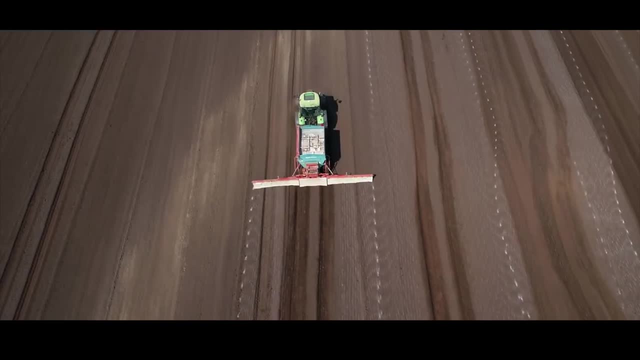 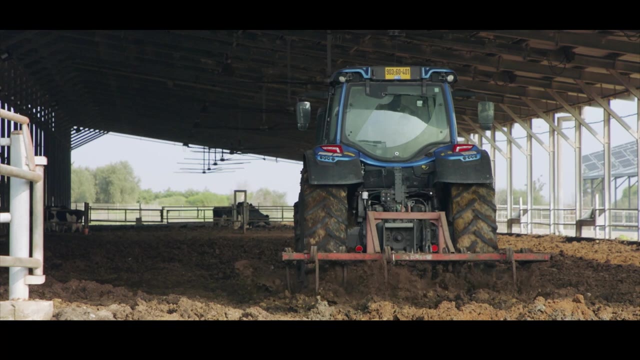 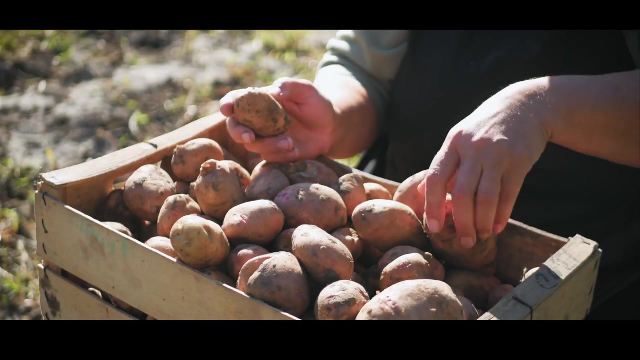 But whether it's because of extreme weather anomalies or improperly regenerated land, the repercussions are the same: More failed and ruined crops. So you see the connection. Poorly managed agricultural and food waste can hurt the land we depend on to grow our food and result in deficient crop yields and even more food waste. 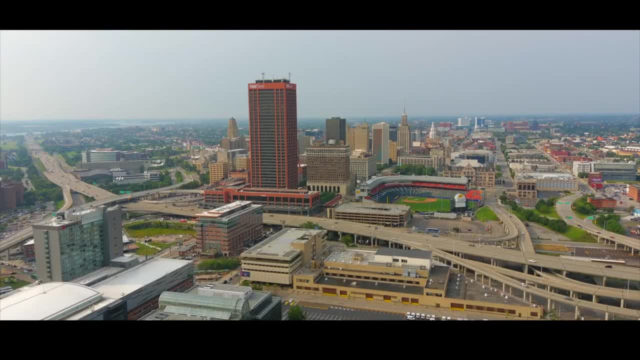 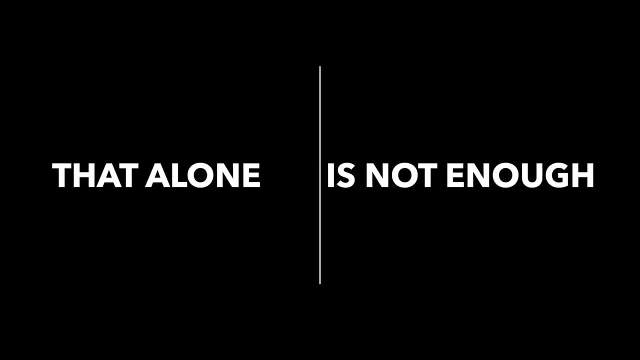 It's a very destructive cycle And while taking advantage of a local or regional food system, it's also a very destructive cycle. So the fact that a local or regional food system is a good way to start scaling back on our carbon footprint, That alone is not enough. 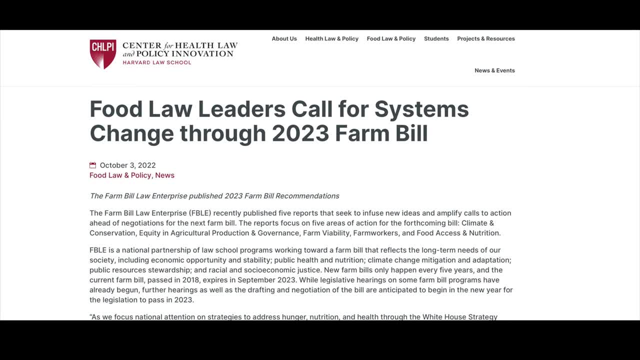 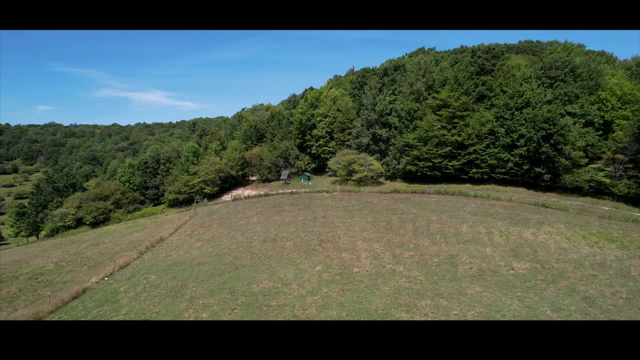 We need to explore all viable options in our efforts to secure a more sustainable, resilient and eco-friendly food system. So let's dive a little deeper into this final component of the food system, as we visit with two farmers who practice what is referred to as regenerative farming. 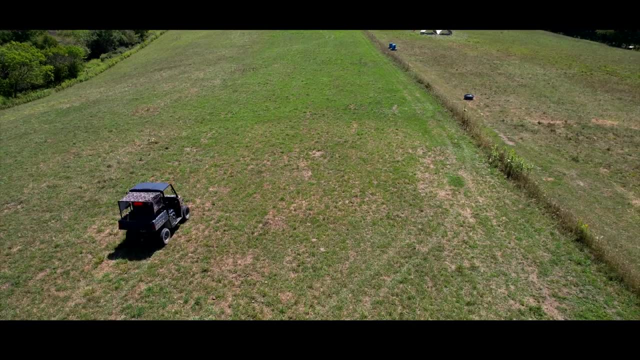 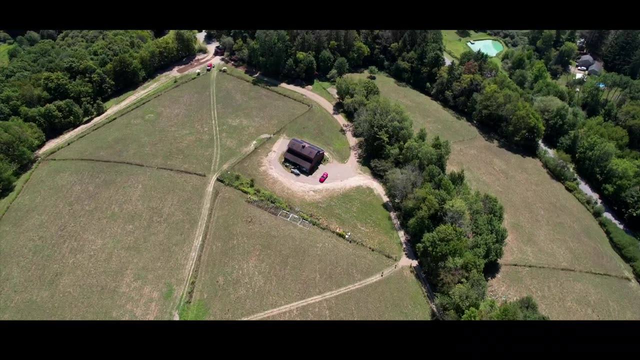 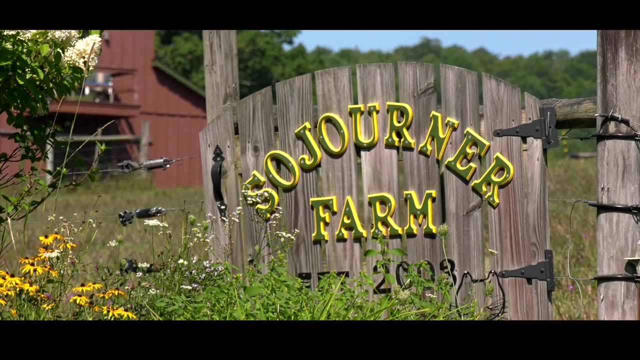 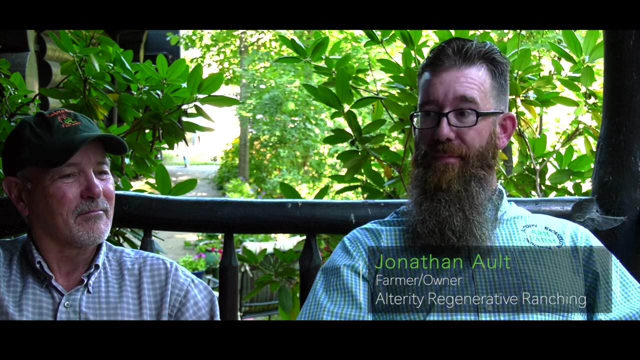 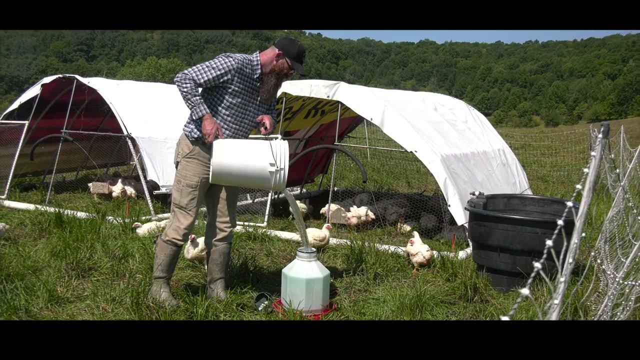 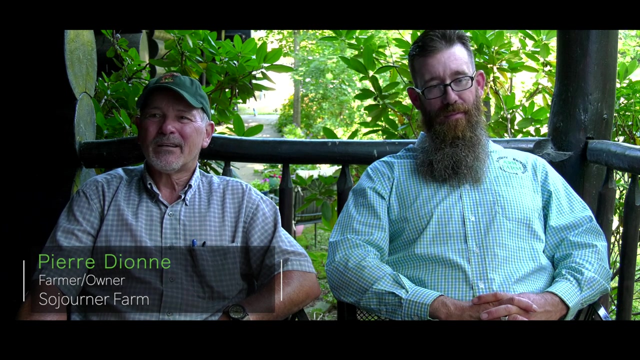 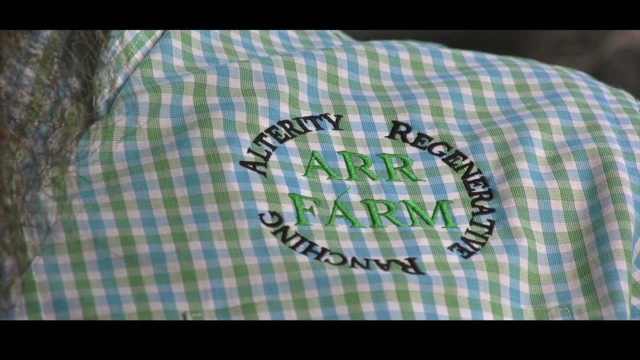 My name is Jonathan Ault. I am a retired city boy And my role on the farm is to help Pierre manage it. My name is Pierre Dion. I'm the owner of Sojourner Farms. I'm a retired physician. What led me to my involvement with regenerative farming is repairing my wife's health. 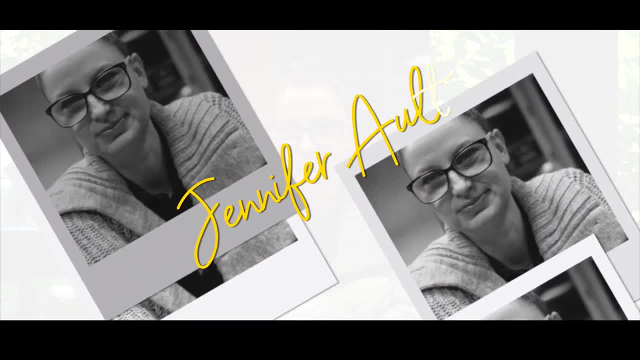 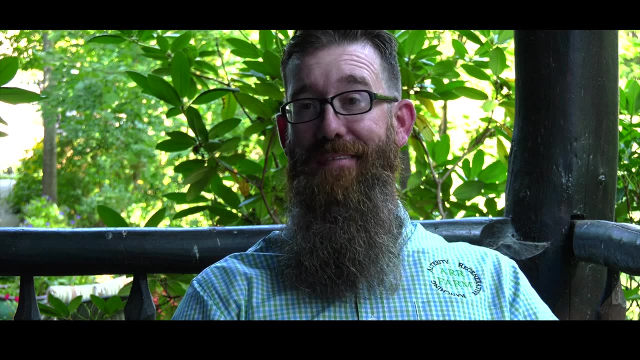 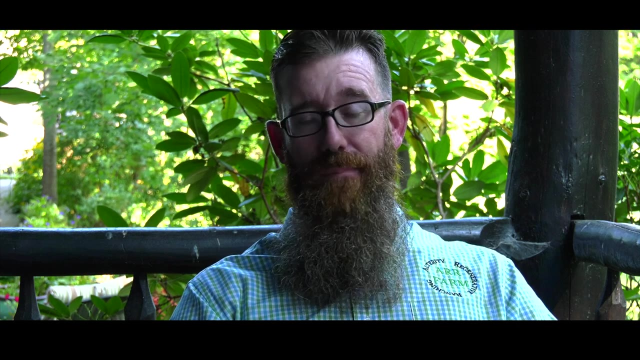 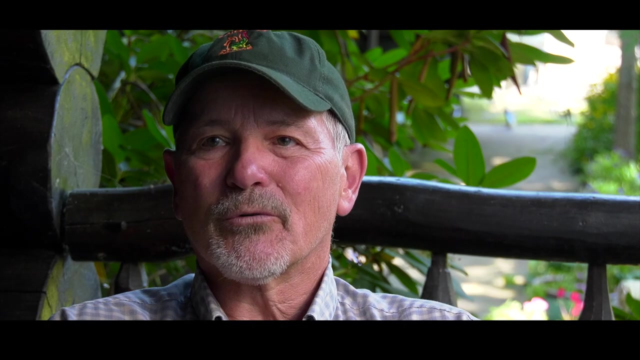 She was diagnosed with Crohn's and after several surgeries and lots of medication she still wasn't healthy. So we changed our diet and got on to clean whole foods and that has made all the difference. I'm from Northern Maine originally and I grew up on a farm, a potato farm, in Northern Maine. 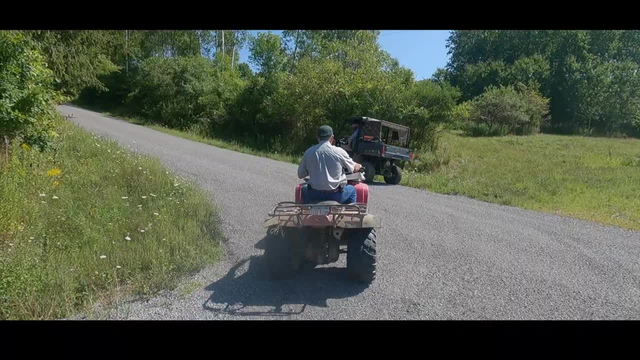 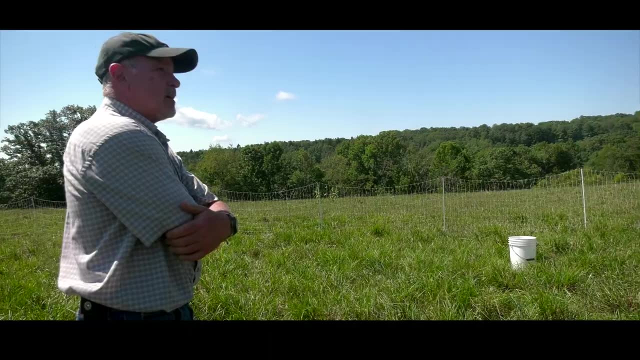 When I first started out it was a hobby and now it's a business, So you look at it from a different perspective if you expect it to at least pay the bills. But I get some enjoyment out of it. It's a problem solving. 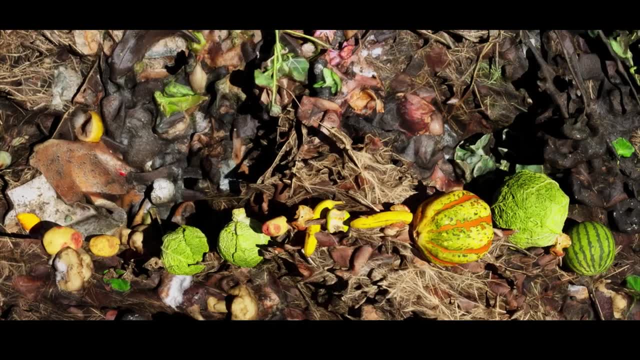 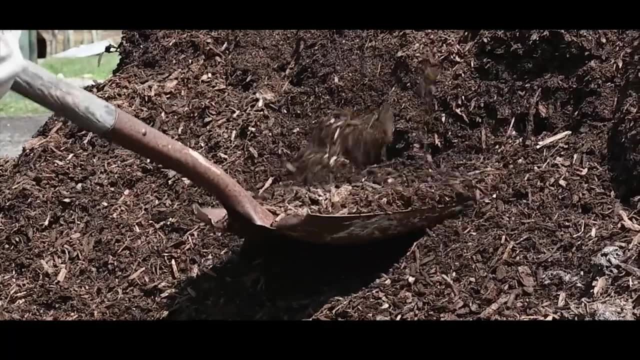 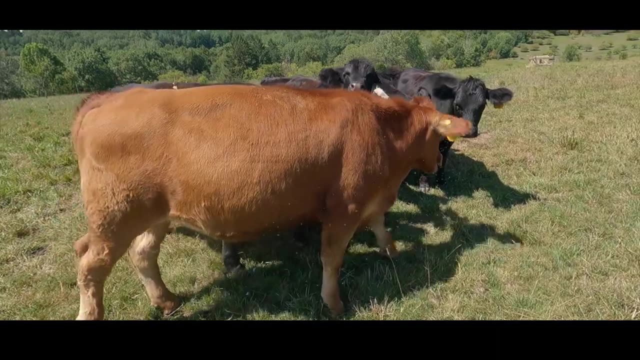 On a regenerative farm there is no waste. We recycle and upcycle anything that will decompose into compost bins or compost piles, and then in the future we will use those on the land Through rotational grazing. we are, in essence, moving our waste around the farm so it can. 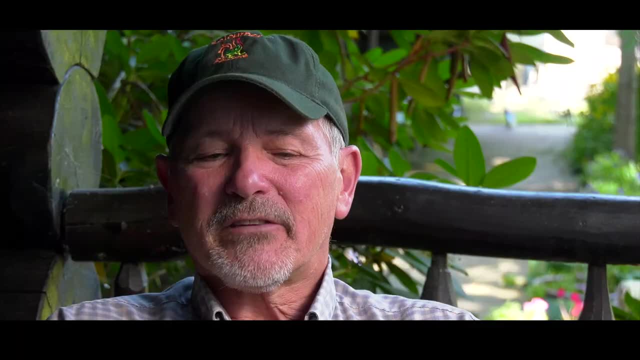 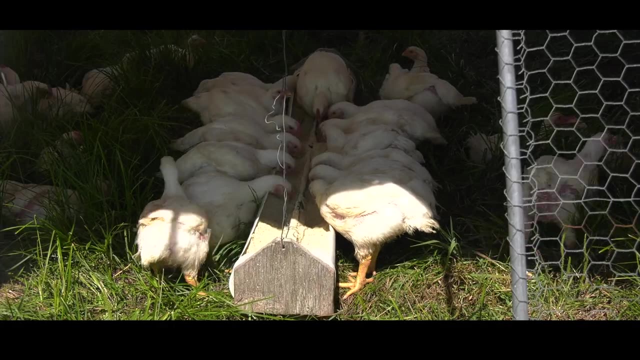 be recycled by the microbiome of the land. I think diversification on the farm is key. It tends to minimize the amount of waste that we have on the farm. It tends to minimize the amount of waste that we have on the farm. It tends to minimize our negative impacts on nature and the environment. and I think regenerative farming to a large degree does that, and having different species of animals helps manage parasites. It allows them to use different types of forages- versus monoculture, where if some disease or bug comes in it can wipe you out If we have issues with one plant. If we have issues with one sector of the farm, The other three or four sectors are probably doing okay and help us through the rough times. basically, Yes, we have been affected by climate change. We have had longer, hotter, drier periods throughout the summer, and what we're doing? 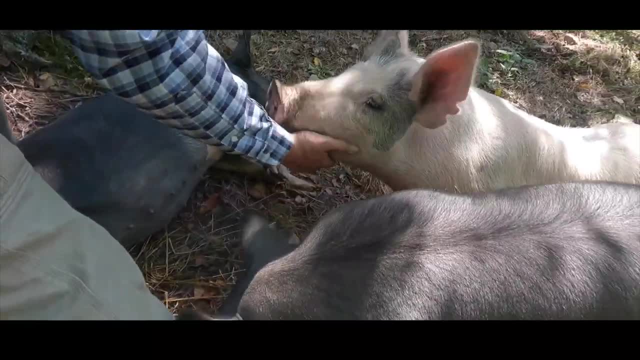 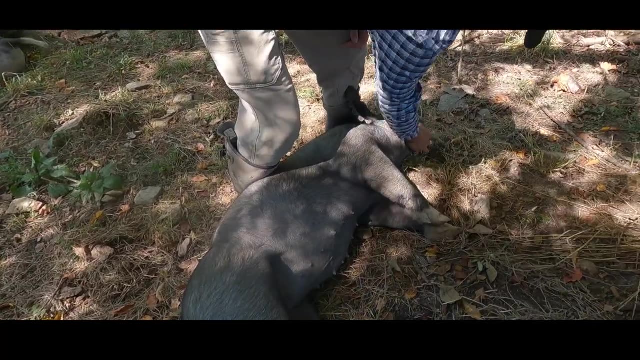 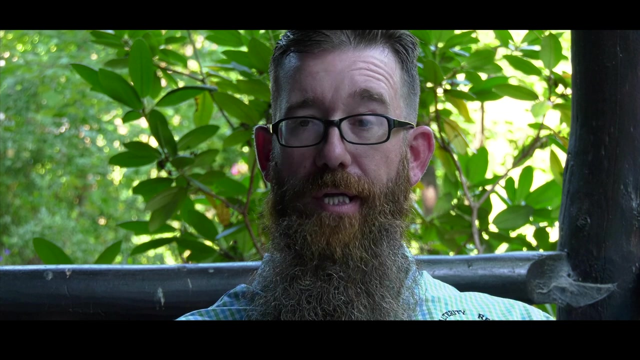 is through observational management. we are changing our strategies. Like in a drought, we'll feed hay and slow the animals down. you know, we basically move the animals as fast as we can. The grass is growing. We're very aware of food waste. 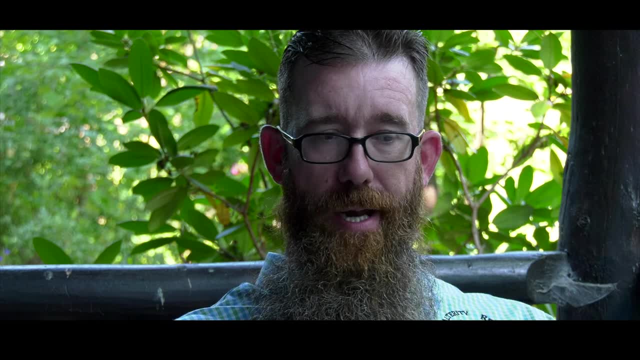 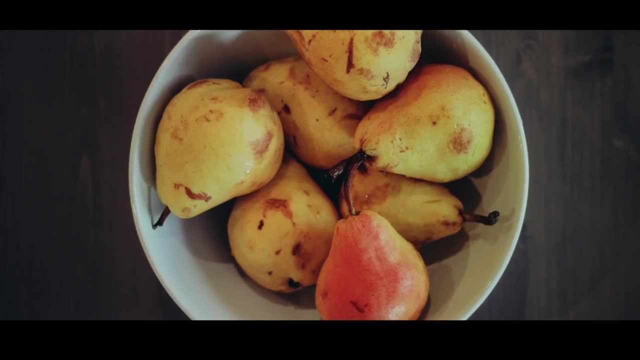 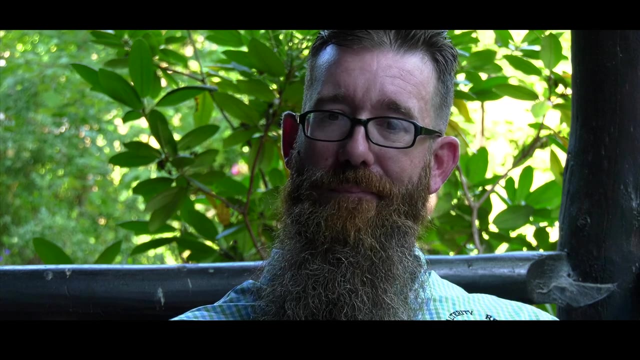 It is disheartening. That's how I feel about it, And how we can deal with it is by not being so superficial, not wanting everything perfect, and also by value adding to these products that aren't the most presentable, by turning them into shelf-stable products. 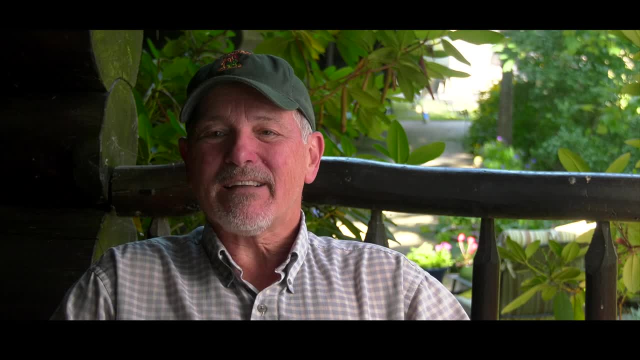 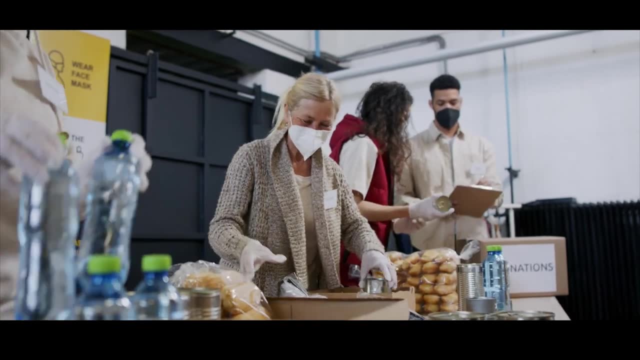 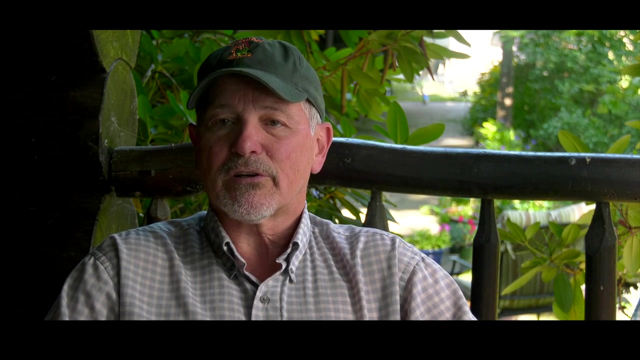 Food waste is a big issue globally. I don't think there's lack of production. There's lack of efficient distribution. basically, We need to pay attention to where the food is going, make sure it's distributed equitably. There shouldn't be any food deserts in this country especially. 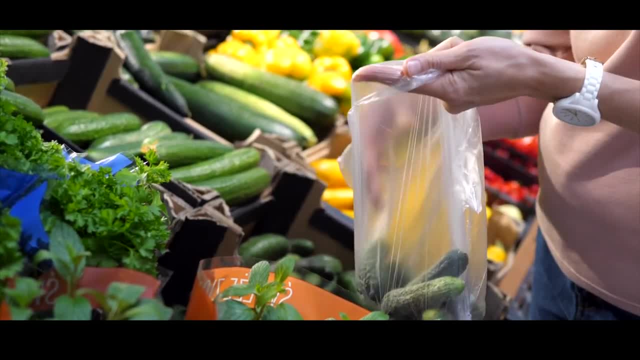 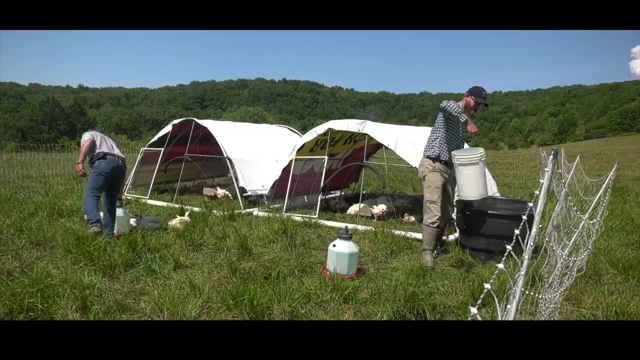 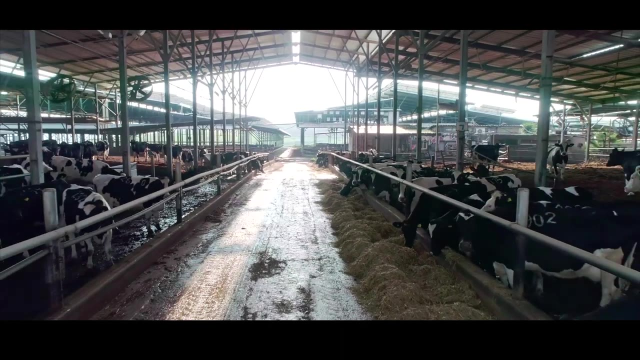 We need to take a step back and start ordering or obtaining our food closer to home. I don't believe there's enough cooperation among farmers. I would love for there to be, but there isn't. One person is saying, hey, we need to create as much as we can in the shortest time as 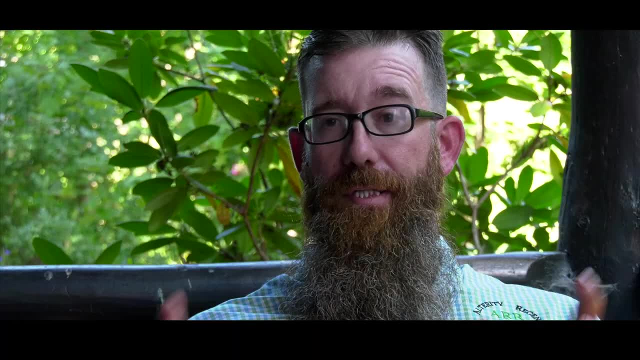 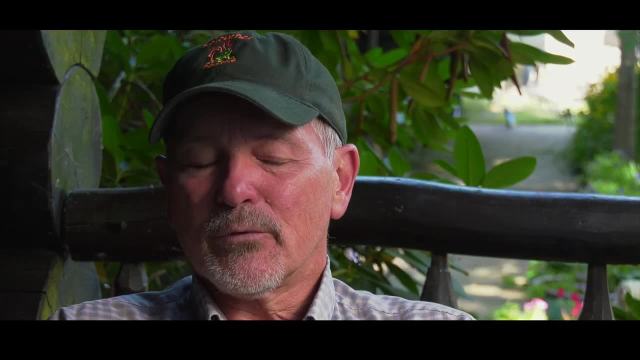 we can, And on the opposing side it would be: we need to create just enough and be environmentally conscious, So those two roads don't always meet. We've done several things on the farm to try to become as carbon neutral as possible. 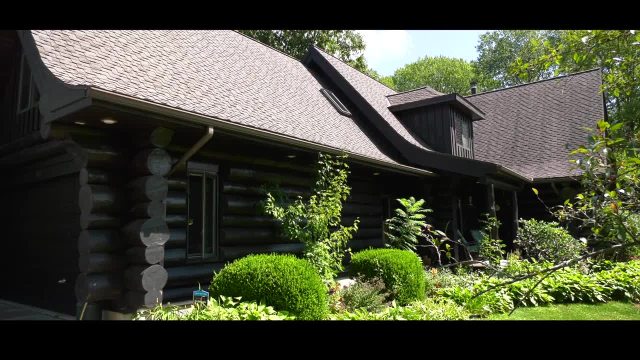 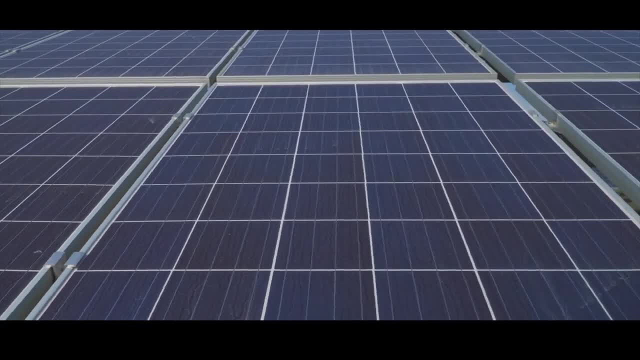 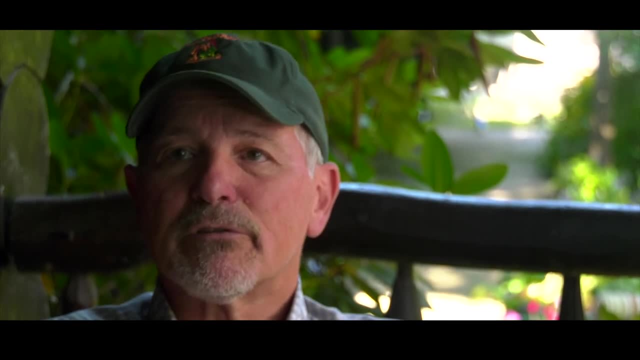 This home that we're in right now used to be heated with fuel oil. We've gone to geothermal and we're we've gone to solar panels. So we're we're still on grid, but we don't pull any electricity from the grid. basically, 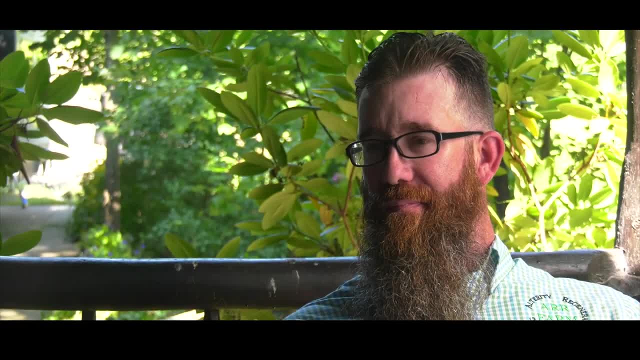 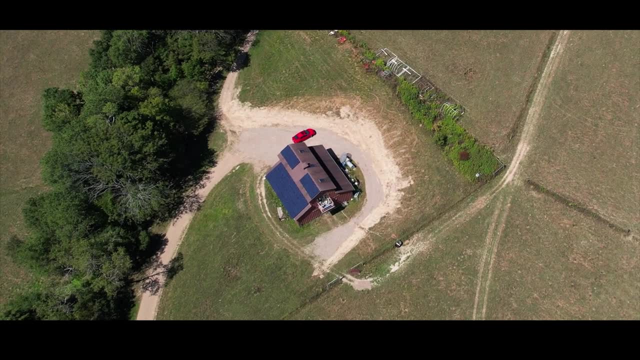 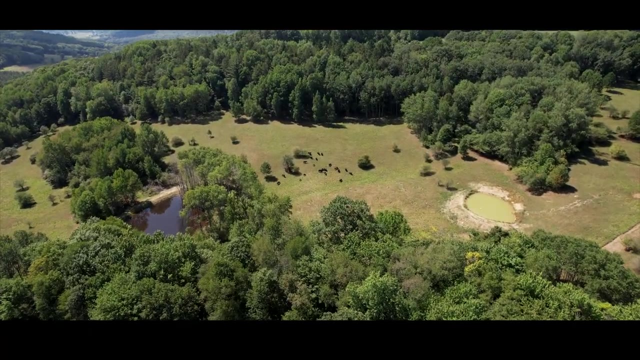 And that's helped create resilience for our home and also for the farm. We have solar panels on one of our barns to run the freezers, the walk-in freezer and refrigerator. We have multiple ponds, but we also have a solar well as as a backup. 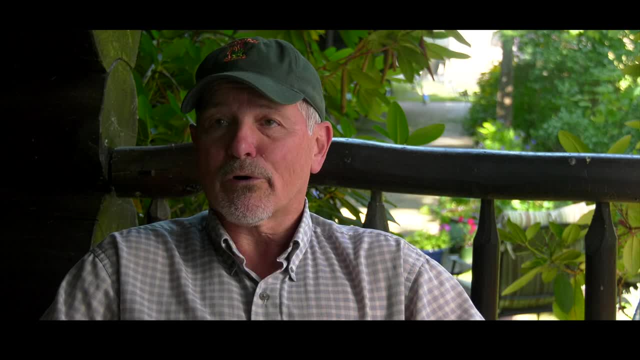 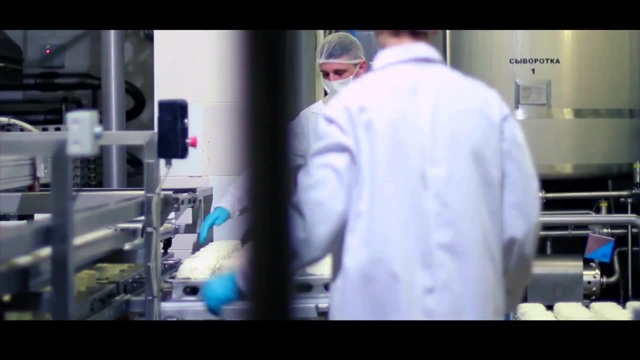 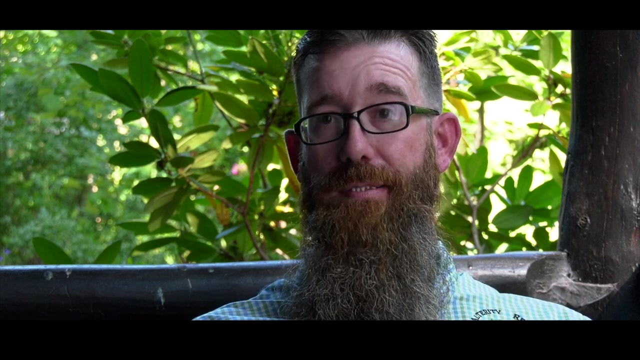 So It basically allows us to diversify our water sources. that, you know, helps us get closer to being carbon neutral. There's only four producers in the country that create bottlenecks to our food system, And if one of those goes out, then everybody panics and shelves are bare. 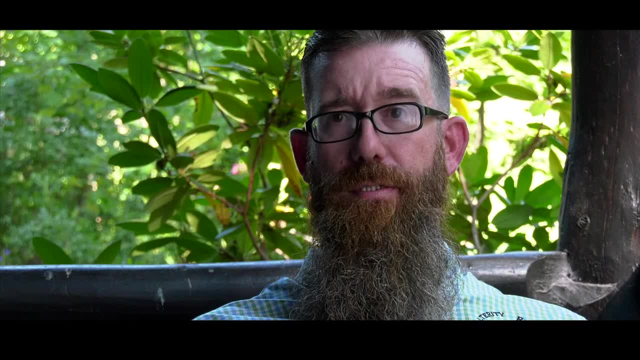 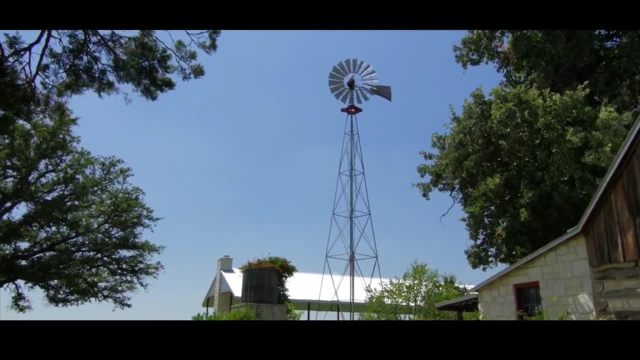 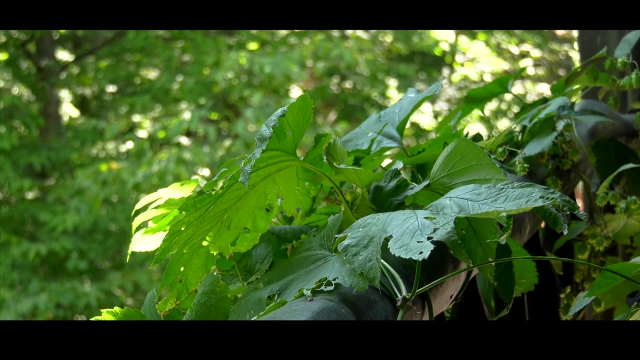 So I believe what we need to do to fix that is to decentralize the food system, make it more community-based and have tens of thousands of these- Okay, Local community driven farms- uh, like ours. There there's niches for everything, but, uh, we need to make the playing field even. 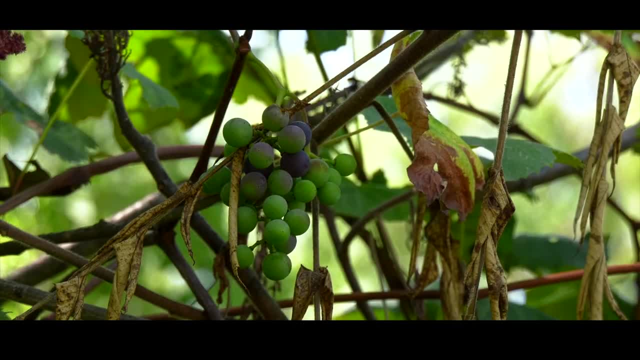 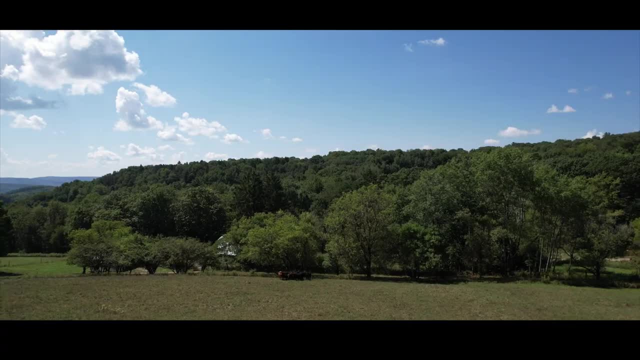 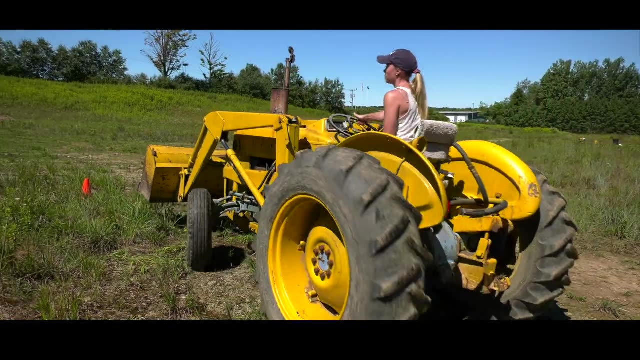 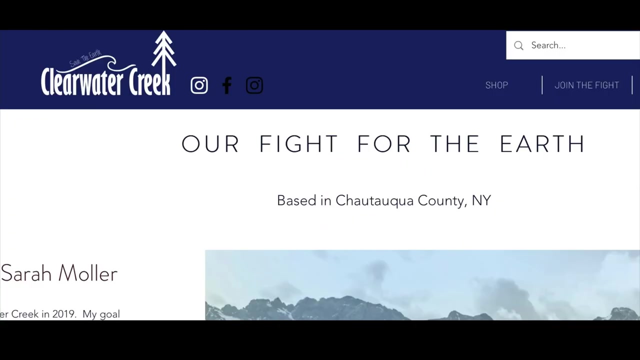 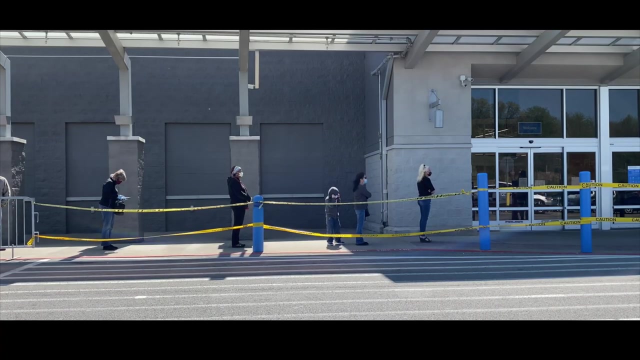 so that small family farms can survive. Okay, Okay, Okay, Okay, Okay. Um, my name is Sarah and I own Clearwater Creek Compost. I started my business one week before the pandemic really hit this country. I didn't think that it would really have much effect, and I was right. 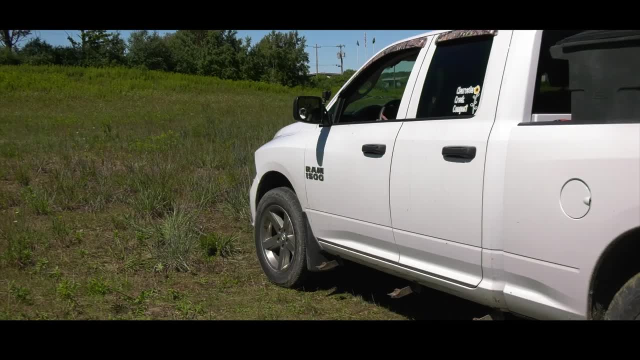 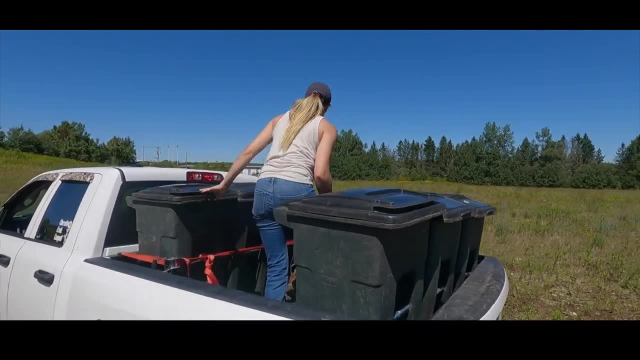 I was able to just continue doing it through it. It's always been important to me to do something positive for the earth And I saw that the only option for food waste and organic waste was the landfill and I thought there's gotta be a better option. 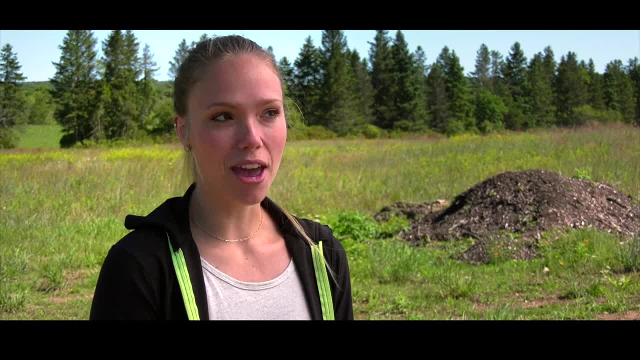 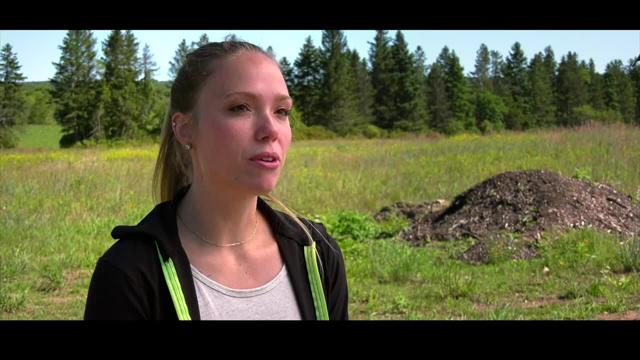 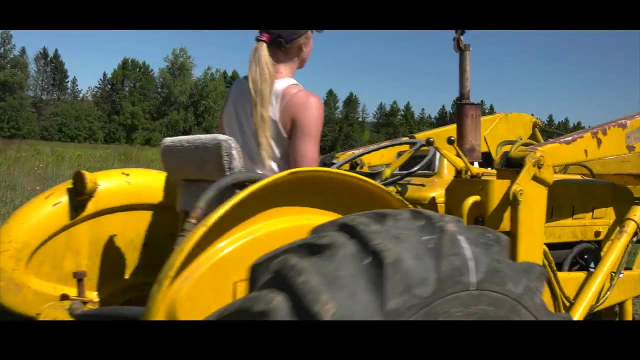 better option and there just wasn't, so I decided to create one and hopefully I set a precedent that other people can follow, and I think that more people have just gotten excited about composting, and that was that's my whole goal this compost business was. it was easy for me to start with very little overhead and 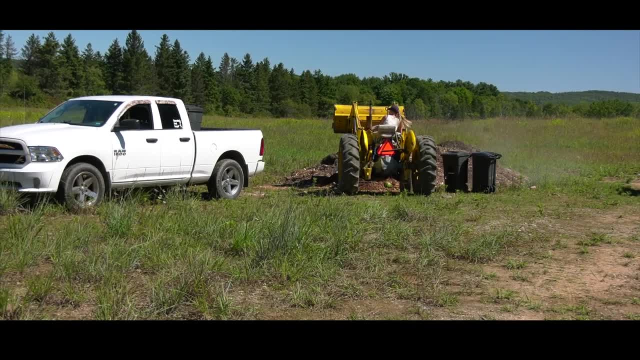 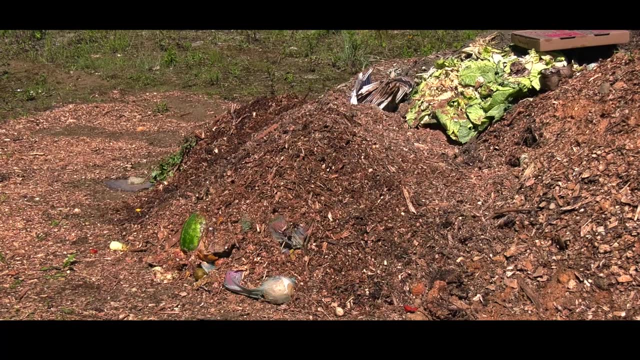 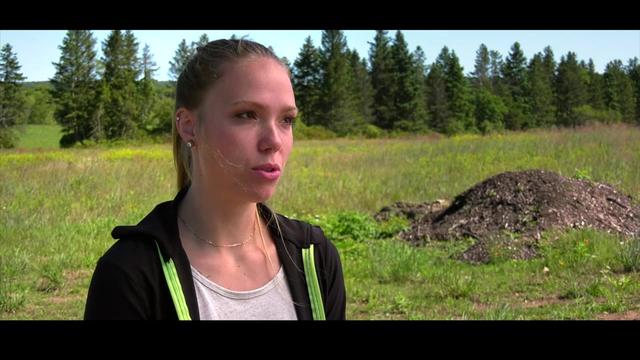 very little investment to get it started and it's been profitable every single year. by composting, we can create healthier food for everybody, we can create a healthier earth and we can reduce our trash and our landfill waste. I do find non compostable items in my compost, yes, so I pick up food scraps. 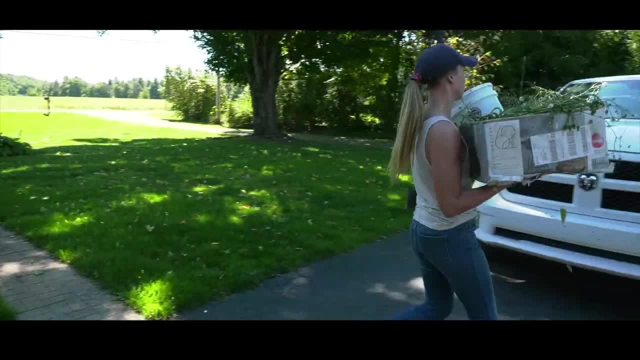 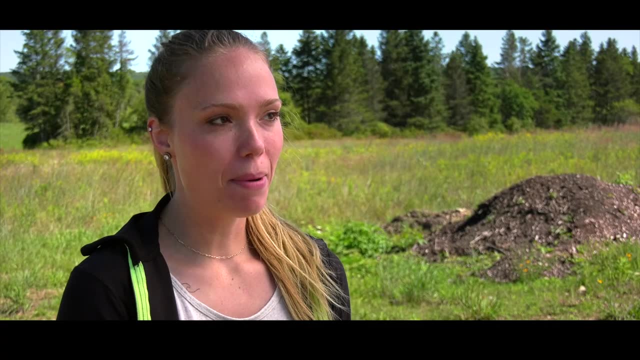 from houses and people are still learning and that's okay. and also kids will throw in a fork or wrappers or something like that, and when I find I might just take them out so to aerate my piles, I use my tractor and I turn the piles. so it's important to get everything that's on the outside to the 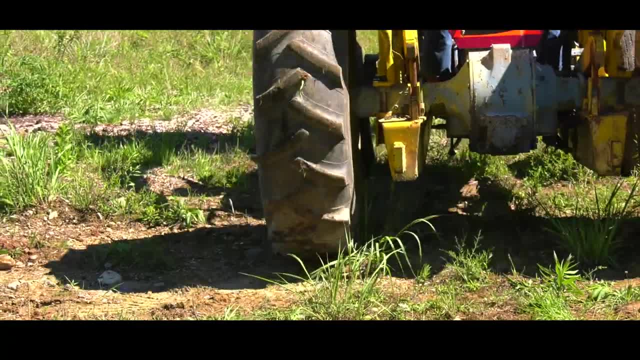 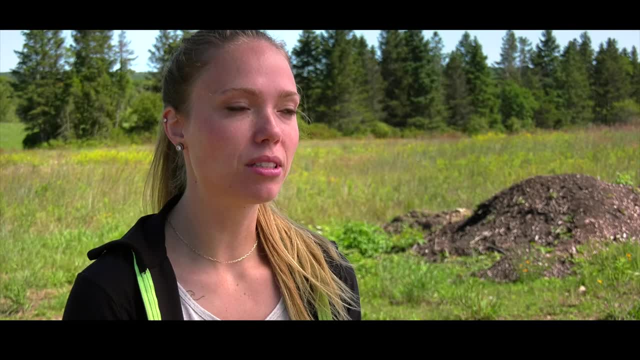 inside and everything it's on the inside out to the outside of the pile and as it's mixing, it's just mixing oxygen with everything. So New York State actually just passed a law, I believe a year ago or two, requiring composting. So they're starting small and 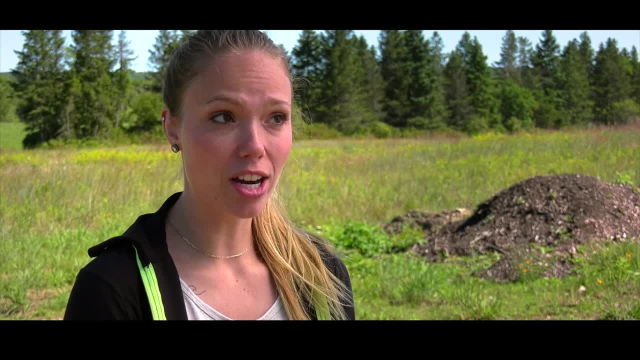 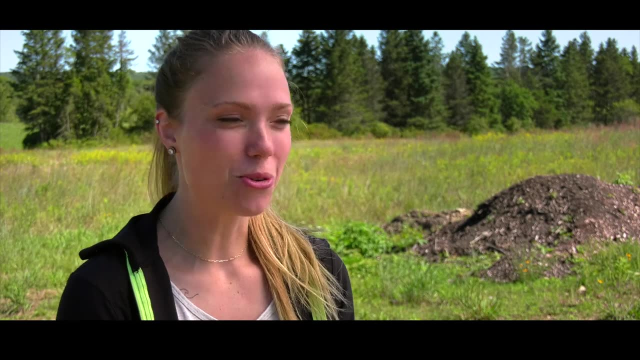 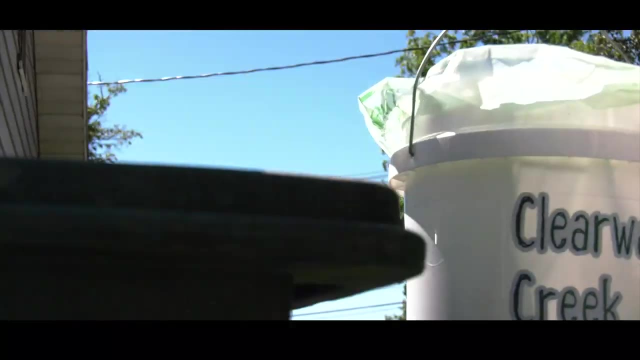 they're starting with a list of businesses that are going to be required to send all their organic material to compost or donate it rather than sending it to the landfill, So that's pretty cool. that's a huge step in the right direction. People have been just really excited to see a compost service pop up. 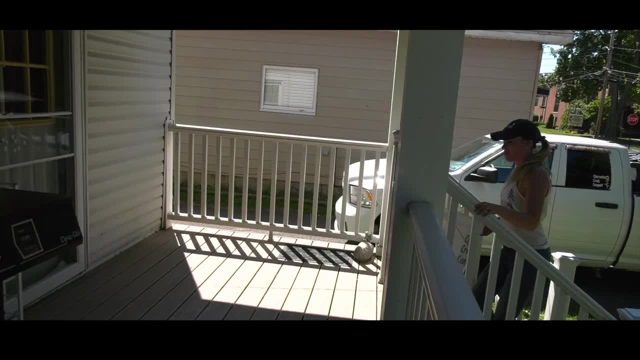 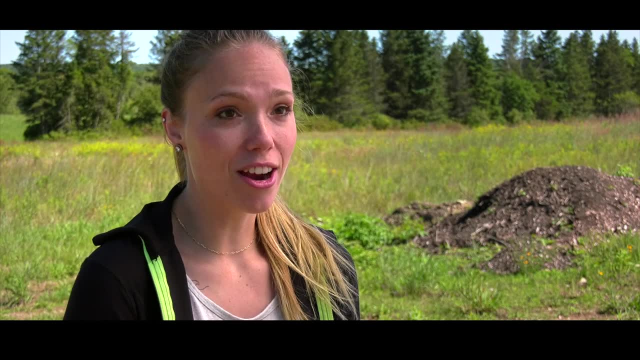 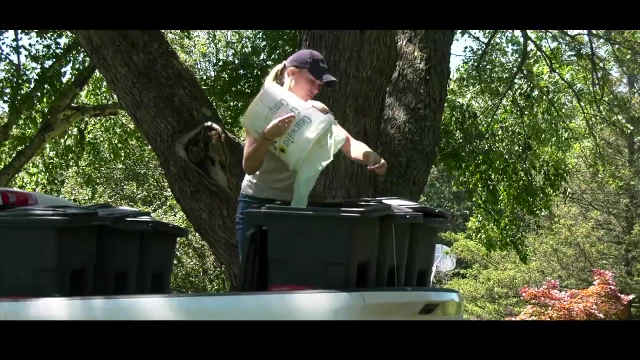 in our area and my customers thank me every single day for picking up their organic waste. And also it's important to know your options. so if you do have a composting service in your area, maybe utilize that, because then you can send your food to back to the earth instead of sending it to the landfill. My pickup 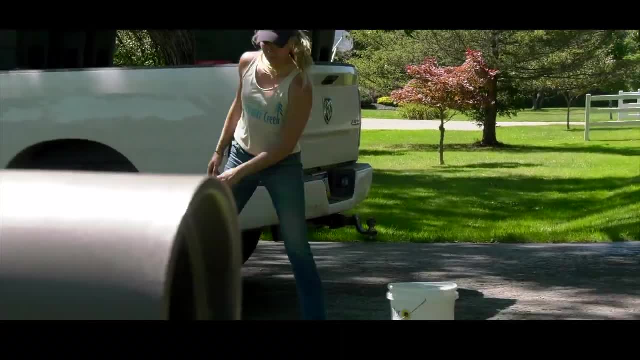 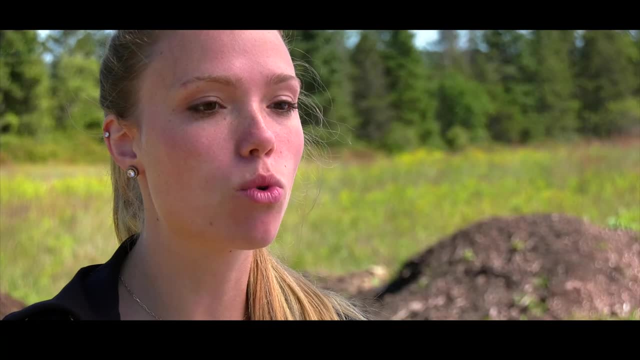 area is about 50 miles in diameter. so just in this one little area we've saved 30,000 pounds of compost. We've saved 30,000 pounds from the landfill and given it all back to the earth. We need to just be more aware of the options for food waste. 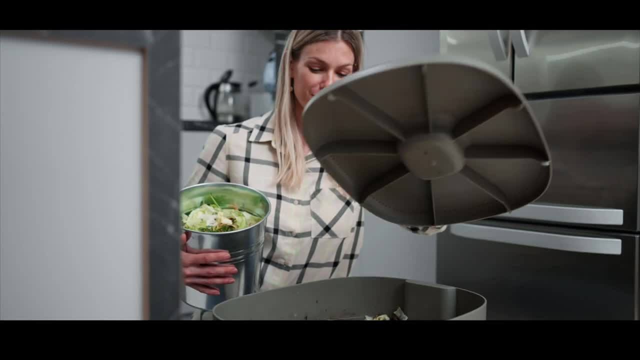 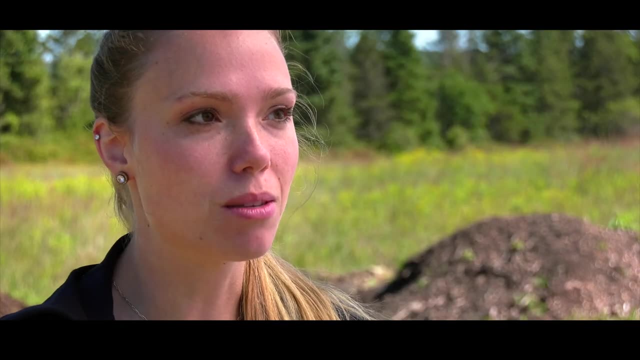 Like. people need to know that they can compost, and you can compost in your own backyard. So I think on every level of the food system there's more options and people need to be aware of those options. The earth is magical, Like composting is. 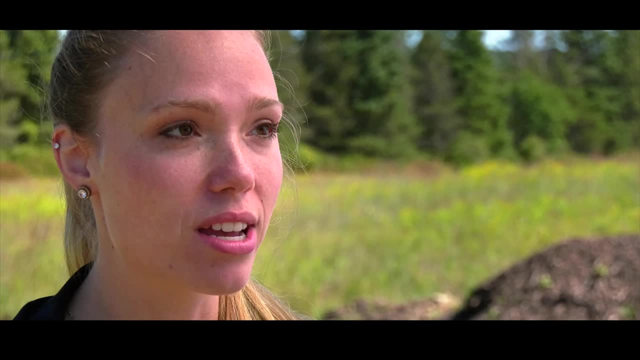 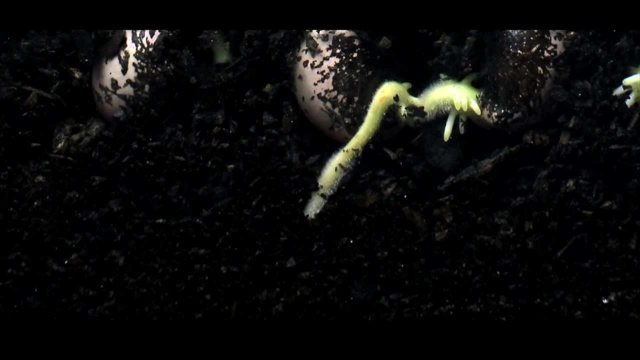 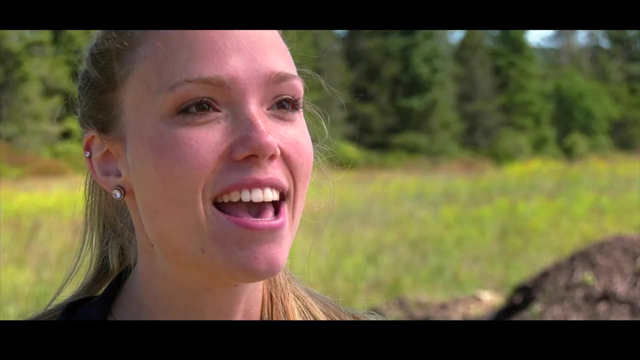 the earth's way of taking organic material and breaking it back down into its very smallest nutrients. and then those very smallest nutrients get to feed other plants and grow other food and nourish more humans and animals and everything And the tiny little microbes and all of the magic that is happening. 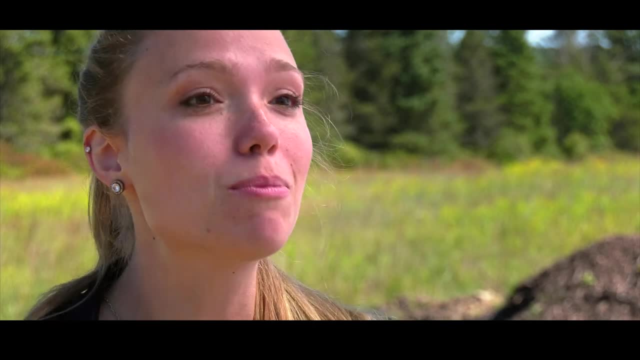 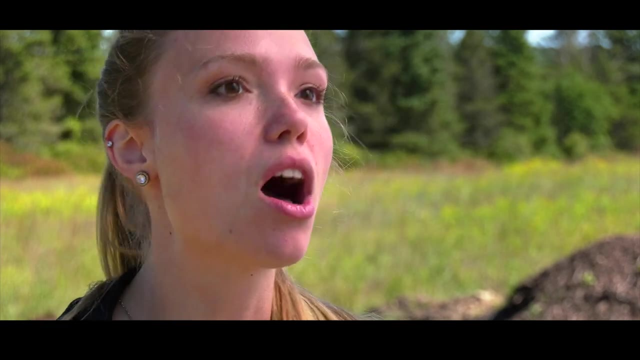 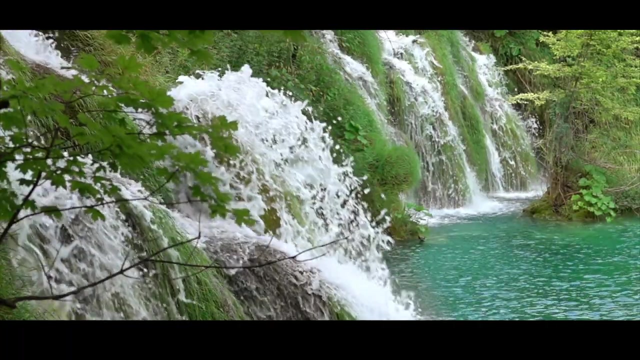 in compost. that's natural to the earth and we need to be utilizing that that process. We need to work with the earth to break down all of our food waste, instead of against the earth and filling the earth with our food waste By a adopting a few new habits and utilizing natural resources in ways that don't. 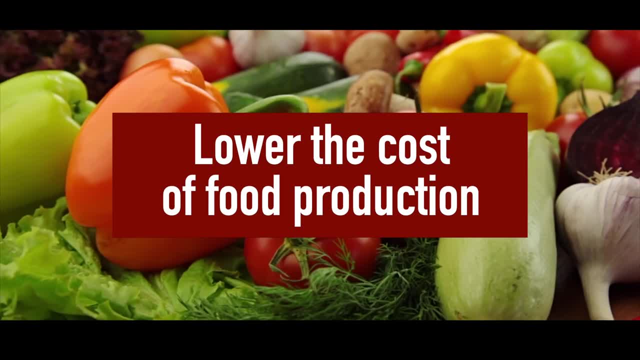 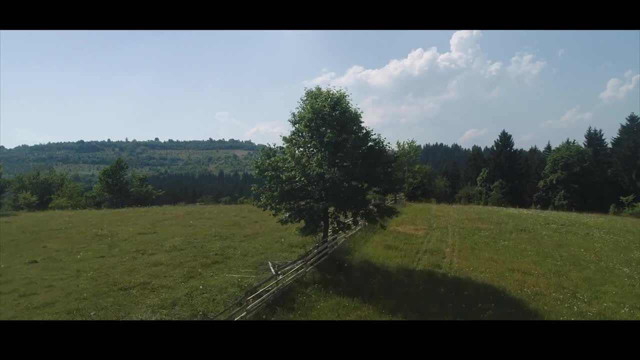 alter the land, we can reduce our impact on the environment, lower the cost of food production, increase energy efficiency and even limit food waste, All while retaining the natural topography of the land for future generations. In a country that has achieved so many amazing things, it is hard to understand. 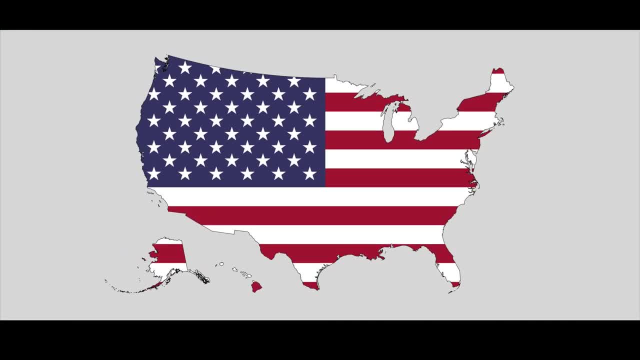 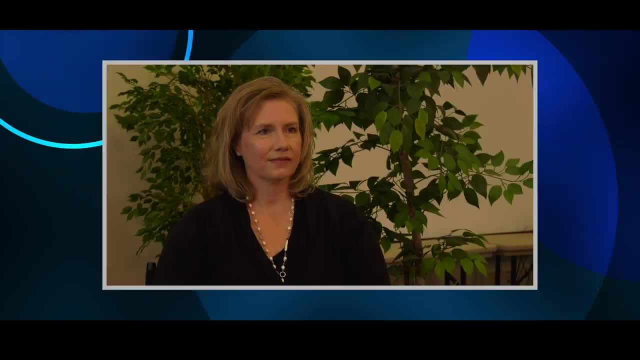 why we can't figure out how to work in unison to save the very things that are keeping us alive. In the final episode of the series, we will try to get a bird's-eye view of everything we have heard so far and explore possible solutions that can lead us to a more resilient food system, while making our 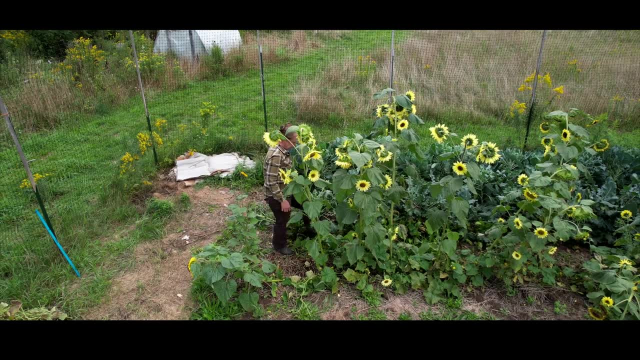 planet safer. So please join us next time for the exciting conclusion to this series. 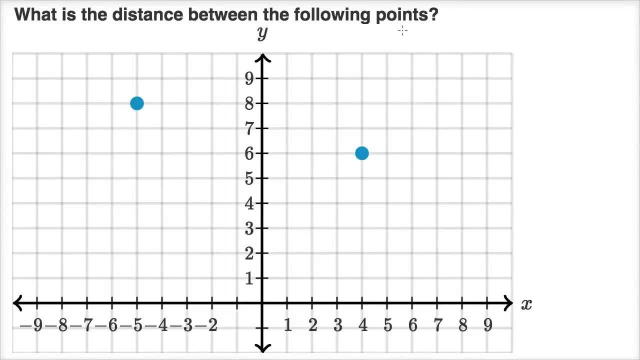 We are asked: what is the distance between the following points? So pause this video and see if you can figure it out. Well, there's multiple ways to think about it. The way I think about it is really to try to draw a right triangle where these points 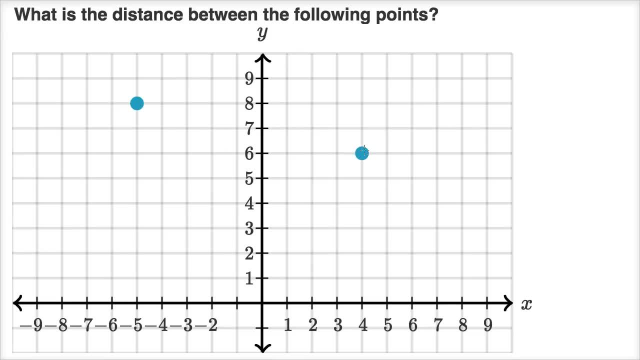 where the line that connects these points is the hypotenuse, And then we can just use the Pythagorean theorem. Let me show you what I am talking about. So let me draw a right triangle here. So that is the height of my right triangle. 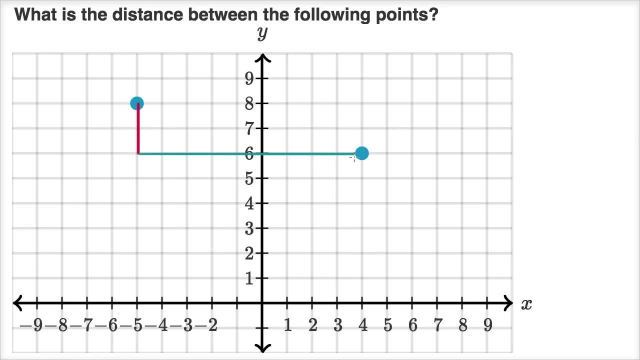 And this is the width of my right triangle, And then the hypotenuse will connect these two points. I could use my little ruler tool here to connect that point and that point right over there. I'll color it in orange. So there you have it.